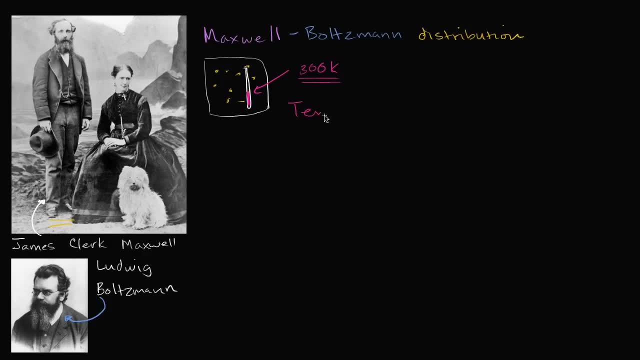 Well, temperature. one way to think about temperature- this would be a very accurate way to think about temperature- is that tempera. I'm spelling it wrong temperature temperature is proportional to average temperature, Average kinetic energy of the molecules in that system. 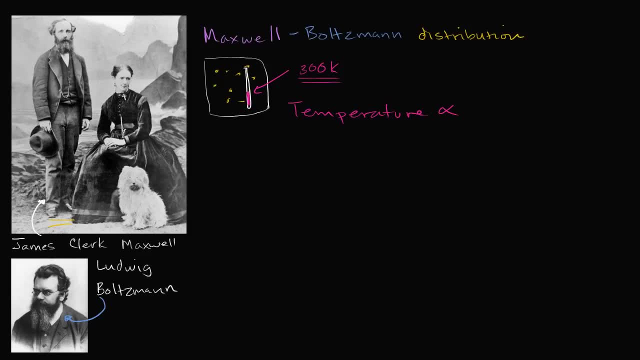 So let me write it this way: Temperature is proportional to average kinetic energy, Average kinetic energy in the system. I'll just write average kinetic energy. So let's make that a little bit more concrete. So let's say that I have two containers. 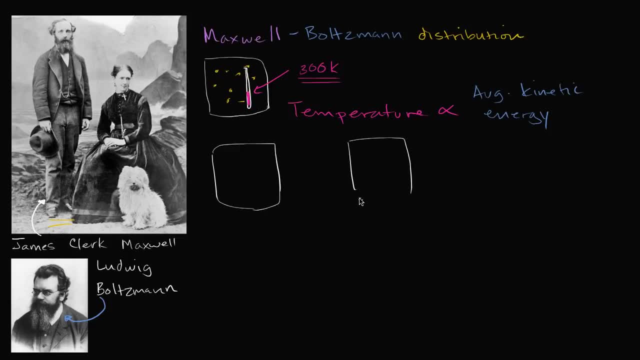 So it's one container And two containers right over here And let's say they have the same number of molecules of nitrogen gas, And I'm just going to draw 10 here. This obviously is not realistic. You'd have many, many more molecules. 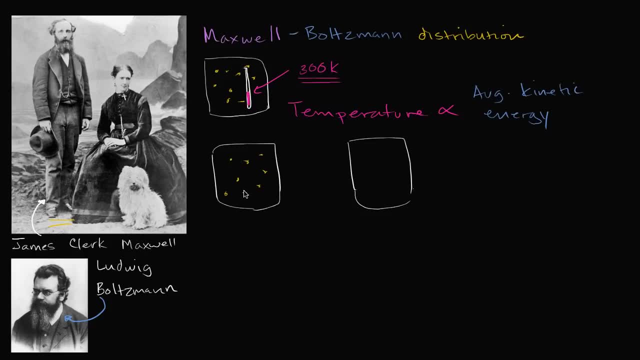 One, two, three, four, five, six, seven, eight, nine, ten. One, two, three, four, five, six, seven, eight, nine, ten. And let's say we know that the temperature here is 300 Kelvin. 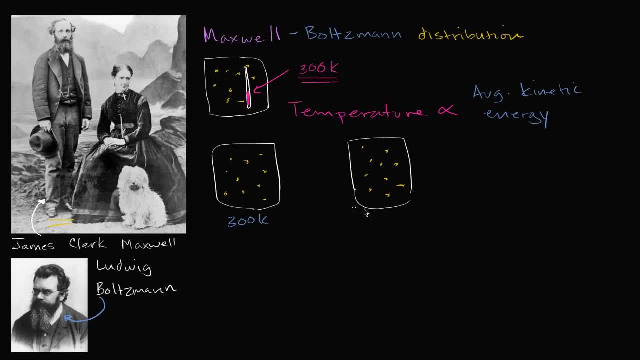 And the temperature. so the temperature of the system is 300.. And the temperature of this system is 200 Kelvin. So if I wanted to visualize what these molecules are doing, They're all moving around, They're bumping. They don't all move together in unison. 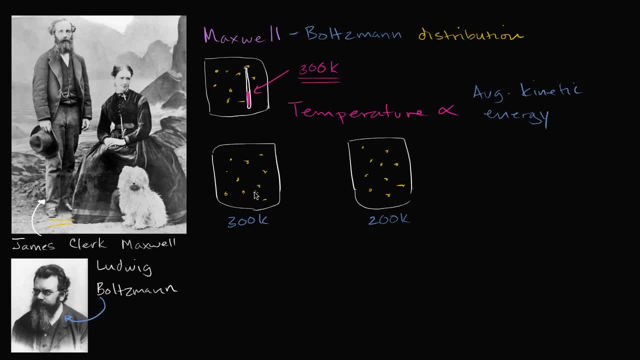 The average kinetic energy of the molecules in this system is going to be higher, And so maybe you have this molecule is moving in that direction. So that's its velocity. This one has this velocity. This one's going there. This one might not be moving much at all. 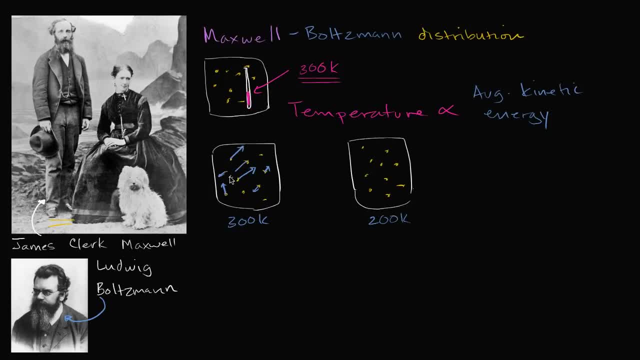 This one might be going really fast that way. This one might be going super fast that way. This is doing that, This is doing that, This is doing that. So if you were to now compare it to this system, This system, you could still have a molecule that is going really fast. 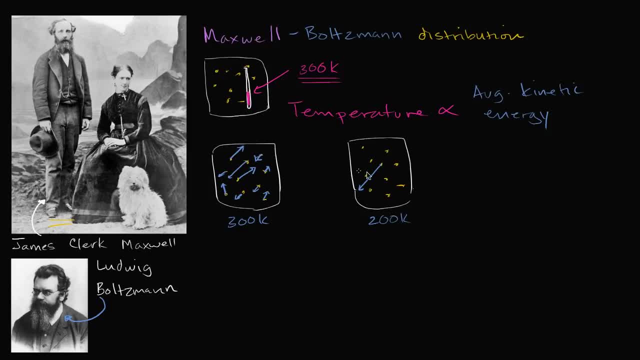 Maybe this molecule is going faster than any of the molecules over here, But on average the molecules here have a lower kinetic energy. So this one maybe, is doing this. I'm going to see if I can draw. on average They're going to have a lower kinetic energy. 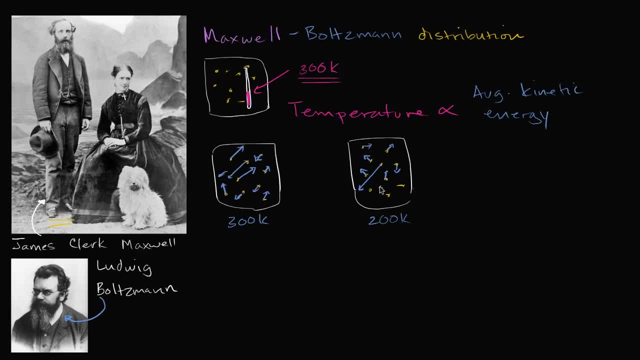 That doesn't mean all of these molecules are necessarily slower than all of these molecules Or have lower kinetic energy than all of these molecules, But on average. on average they're going to have less kinetic energy And we can actually draw a distribution. 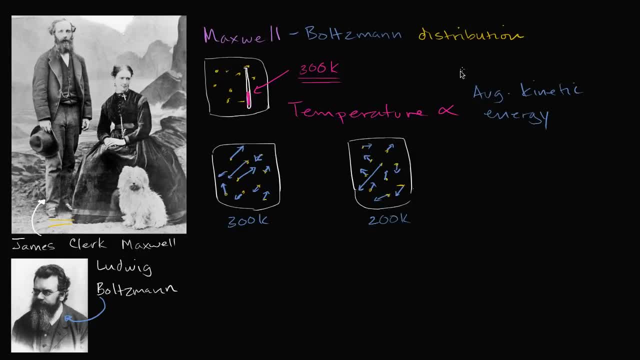 And this distribution, that is the Maxwell-Boltzmann distribution. So if we let me draw a little coordinate plane here, So let me let me draw a coordinate plane, So if on this axis I were to put speed, If I were to put speed, 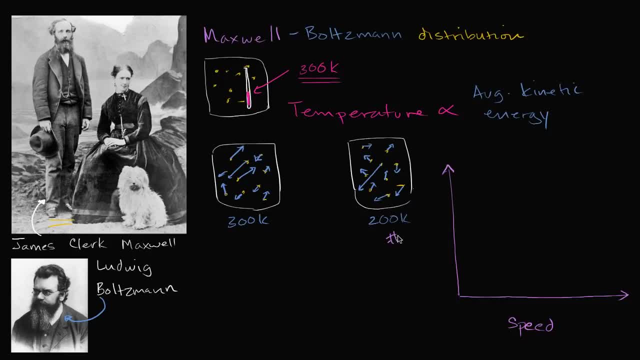 And on this axis I would put number of molecules, Number of number of molecules, Right over here. For this system, the system that is at 300 Kelvin, The distribution might look like this. So it might look, the distribution. 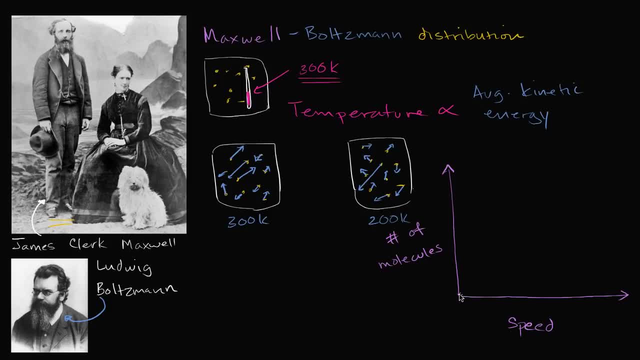 Let me do this in a new color. So the distribution, This is going to be all of the molecules The distribution might look. might look like this, Might look like this, And this would actually be the Maxwell-Boltzmann distribution for this system. 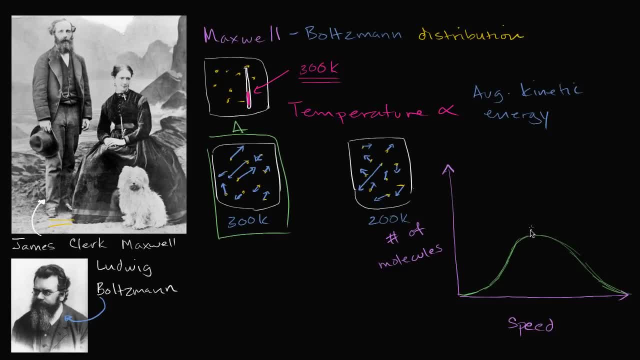 For a system. let's call this system A System A Right over here. And this system that has a lower, that has a lower temperature, Which means it also has a lower kinetic energy, The distribution of its particles. So the most likely, the most probable, 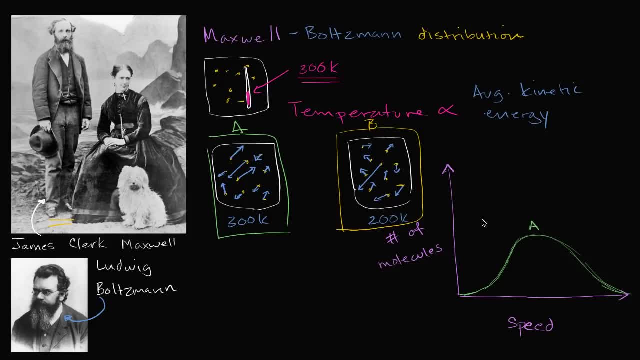 You're going to have the highest number of molecules at a slower speed. Let's say you're going to have it at this speed, right over here. So its distribution, Its distribution, might look something like this Now. So it might look something like that: 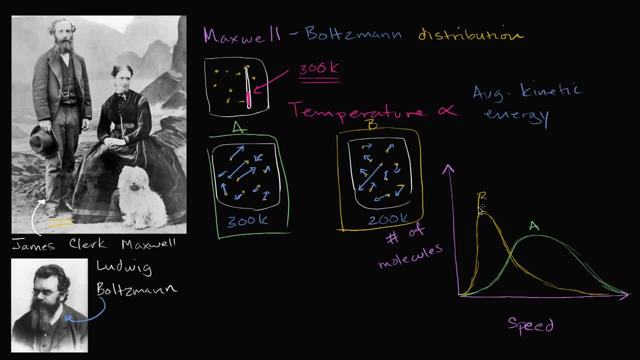 Now why is this one? It might make sense to you that, okay, the most probable, The speed at which I have the most molecules I get that that's going to be lower than the speed at which I have the most molecules in system A. 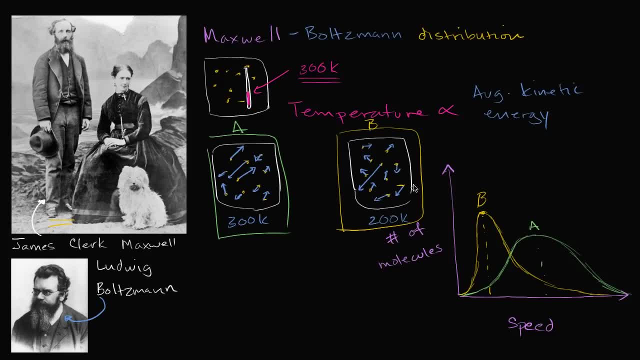 Because I have? because these, on average, these things have less kinetic energy. They're going to have less speed. But why is this peak higher? Well, you got to remember we're talking about the same number of molecules. So if you have the same number of molecules, 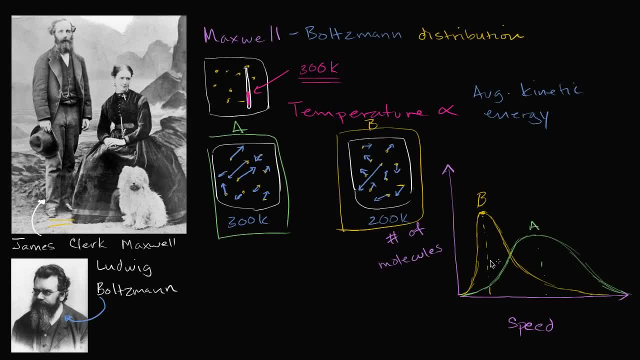 That means that the areas under these curves need to be the same. So if this one is narrower, it's going to be taller. And if I were going to, if I were to somehow raise the temperature of this system even more, Let's say I create a third system. 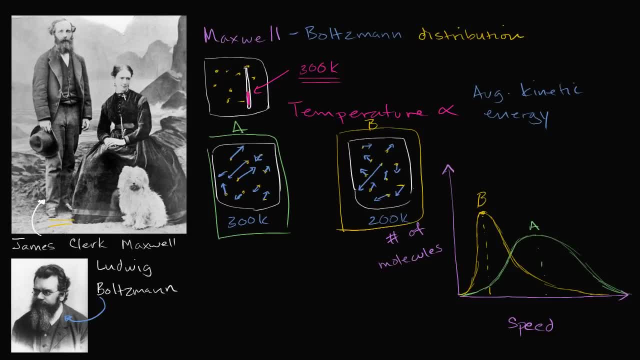 Or I get this, or let's say I were to heat it up to 400 Kelvin. Well then, then it would look, then my distribution would look something would look something like this: So this is if I, if I heated it up. 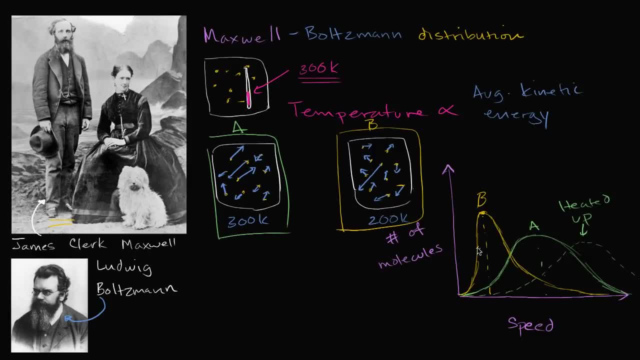 Heated, heated up, And so this is all the Maxwell-Boltzmann distribution is. I'm not giving you the the more involved hairy equation for it, But really the idea of what it is, And it's a pretty neat idea. 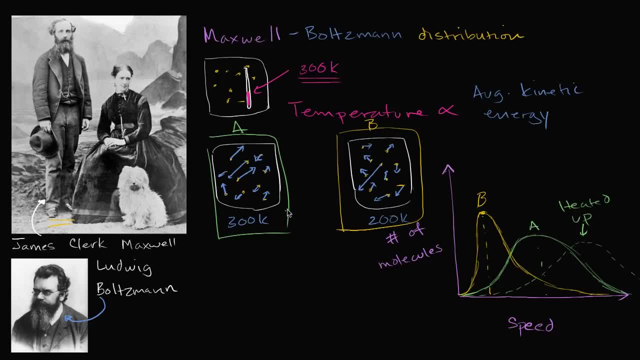 And actually, when you actually think about the actual speeds of some of these particles, Even in the air around you, The air around you It looks, it looks pretty stationary to me, But it turns out in the air around you is mostly nitrogen. 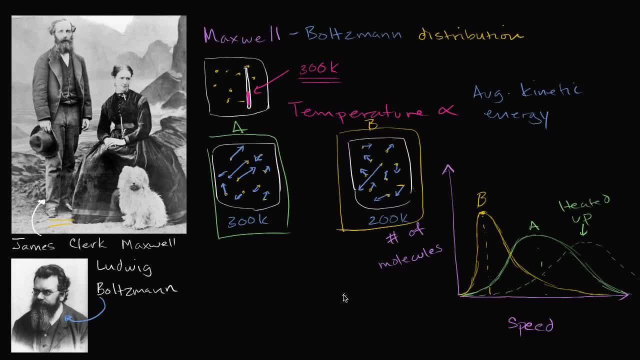 That the most the most probable speed of if you picked a random nitrogen molecule around you right now. So the most probable speed- I'm going to write this down because this is pretty mind blowing- Most probable speed at room temperature. Probable prob probable speed. 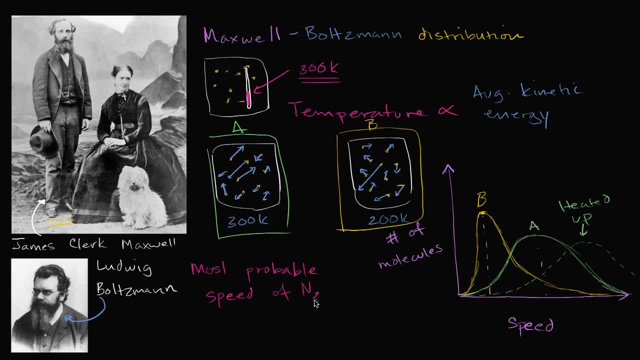 Speed of N2 at room temperature. Room temperature Temperature. So let's say that this was the Maxwell-Boltzmann distribution for for nitrogen at room temperature. Let's say that that's let's say we make. we call room temperature 300 Kelvin. 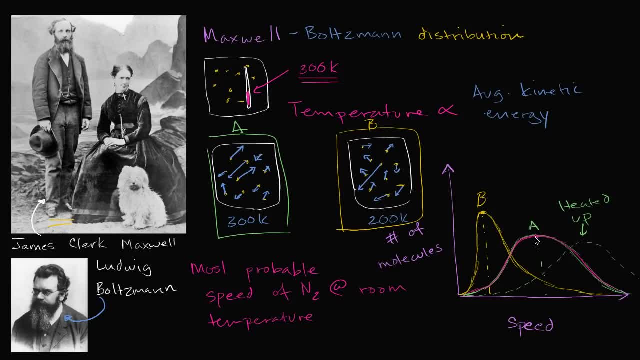 This most probable speed right over here, The one where we have the most molecules, The one where we're going to have the most molecules at that speed. In fact, guess what that is going to be before I tell you, Because it's actually mind boggling. 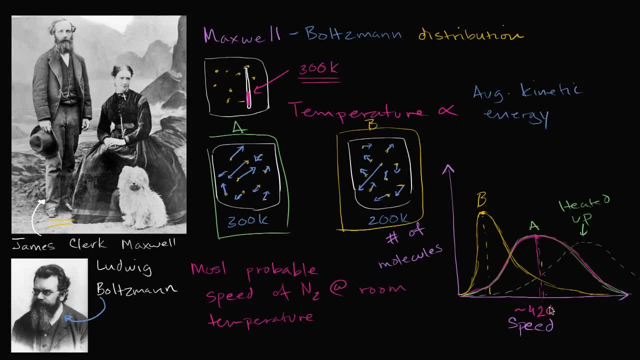 It turns out that it is approximately 400, 400 and actually, at 300 Kelvin it's going to be 422 meters per second. 422 meters per second. Imagine something traveling 422 meters in a second, And if you're used to thinking in terms of miles per hour, 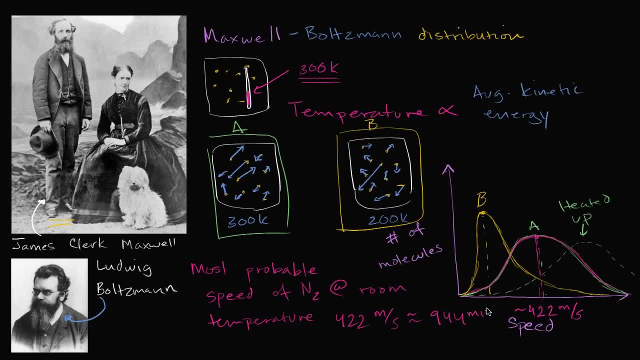 This is approximately 944 miles miles per hour. So right now around you You have actually The most probable, the highest number of the nitrogen molecules around you Are traveling at roughly this speed And they're- they're bumping into you.